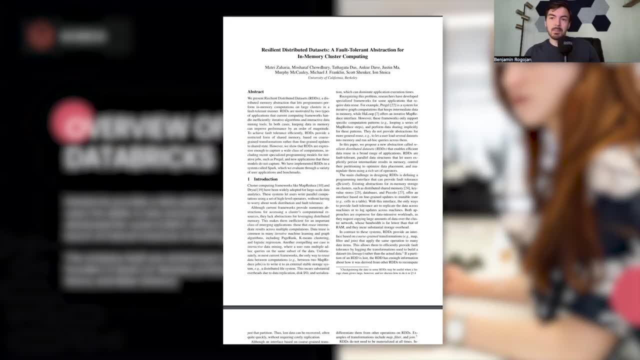 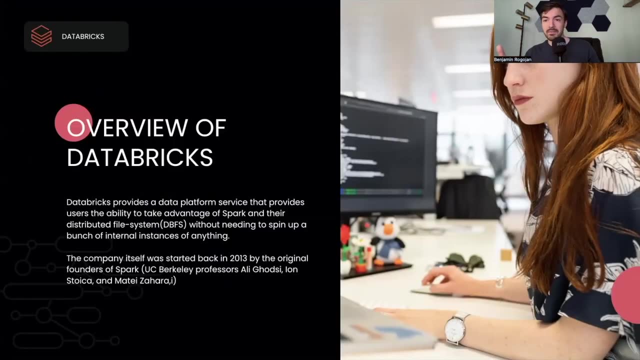 It's basically processing and what you're often going to hear is RDDs. I'm going to put up the paper here as well- Link For anyone who's interested in learning more. But basically it was developed by some professors at UC Berkeley and eventually, like anything else, that is difficult to manage. 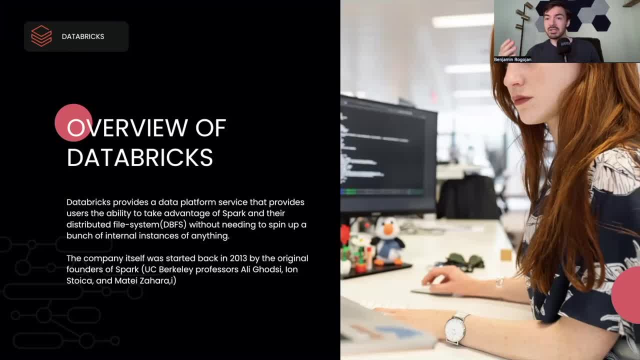 people eventually wanted an option for managed Spark services. If you're familiar with AWS, EMR or GCP's Dataproc, that's essentially what you could do. You could set up Spark jobs using those managed services. But what if you went a few steps further? 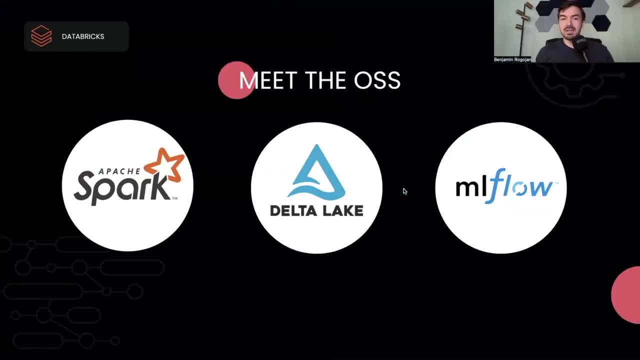 That's where Databricks comes in. Databricks is not just one open source solution, but in fact it's multiple. At its core, in particular, it's Spark, Delta Lake and MLflow. In particular, Spark is pretty much unavoidable. 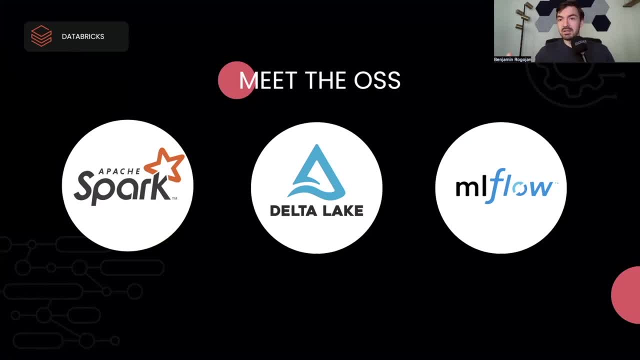 You're going to use it whenever you're processing data. Delta Lake can set up Delta tables, So that's something that we can dive into in a second video, And MLflow, again, is more of an option for those of you who haven't worked with MLflow. 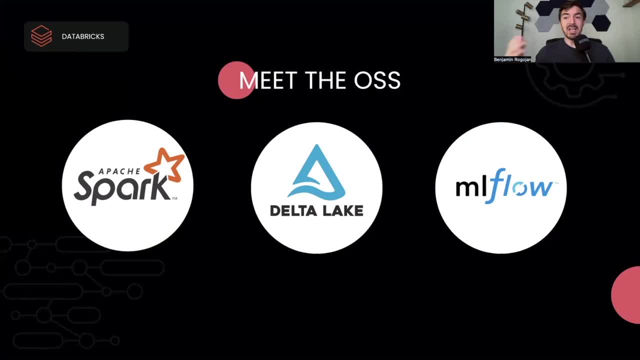 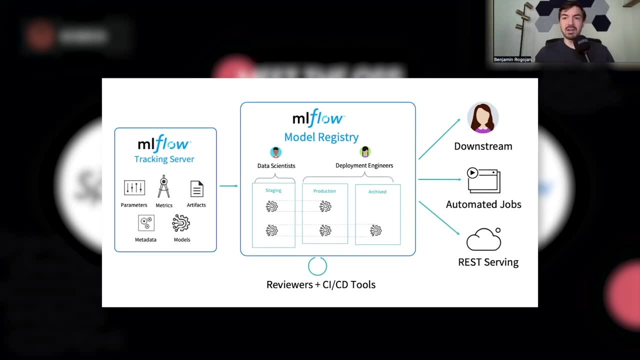 It's basically going to take a lot of those questions You have if you're a data scientist in terms of how do I deploy this model. That's going to be your answer for a lot of people. It's going to take care of model registry, model deployment, some model monitoring. 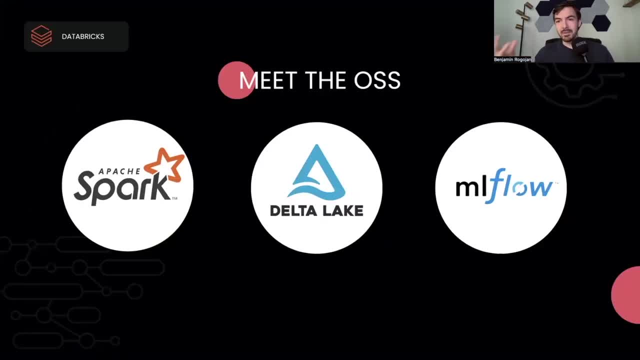 A lot of these things that we don't always know what to do with. You're like: I've developed a model. Now what do I do with it? MLflow is one option. Another option you might have heard of is Kubeflow. 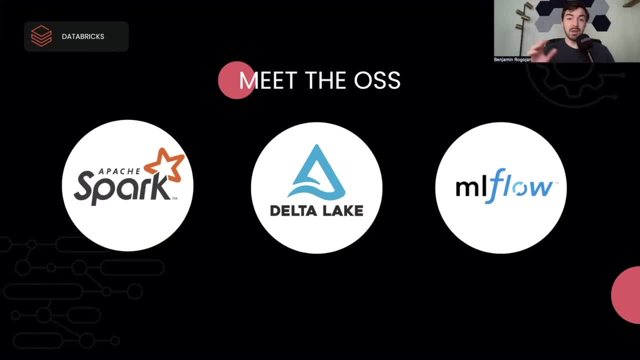 So MLflow is what Databricks uses, as well as, again, Delta Lake and Spark. But again, most people are going to most likely interact with the Spark layer mostly, but in a way that is very friendly for any data scientist or data engineer, because they've set it up in such a way. 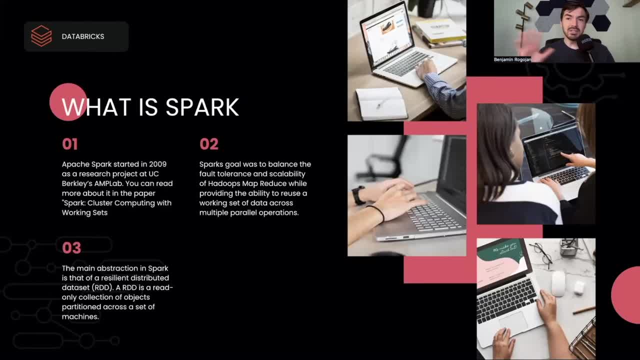 that if you're familiar with Jupyter Notebooks, you're going to do great. So let's just dive into Spark really lightly so you can kind of understand what it is, what it's doing and what's the whole focus. what is an RDD? 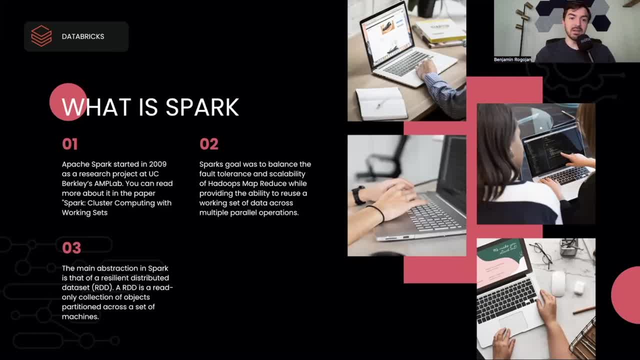 So Apache Spark was started in 2009 at UC Berkeley at AMP Labs, with the goal of balancing fault tolerance and scalability that often you find with Hadoop in a solution, and the goal of Spark was to balance the fault tolerance and scalability of Hadoop while also providing that ability to essentially 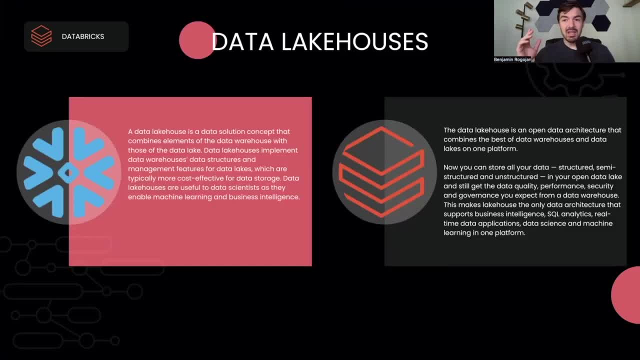 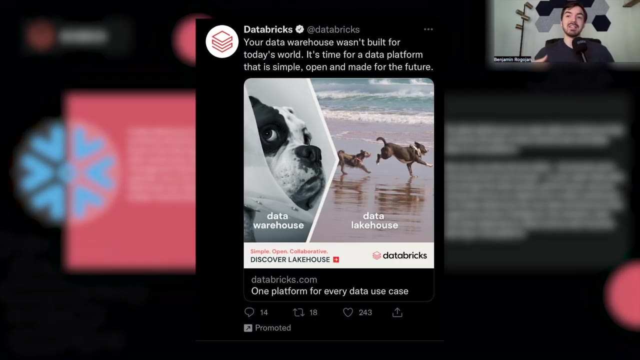 reuse sets of data across multiple processes. Now I think it would be a miss if I didn't go over data lake houses, because clearly Databricks has decided to bet on this horse And basically every ad I've ever seen for Databricks is often poking fun at the concept of a data warehouse. 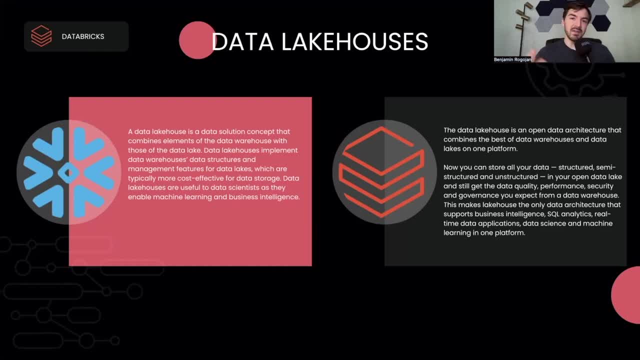 Because what they are viewing in terms of the future of development and data management isn't a data warehouse, but instead a data lake, and both Snowflake and Databricks have their definitions in terms of what is a data lake house. If you ask Snowflake what is a data lake house, they're going to define it again. 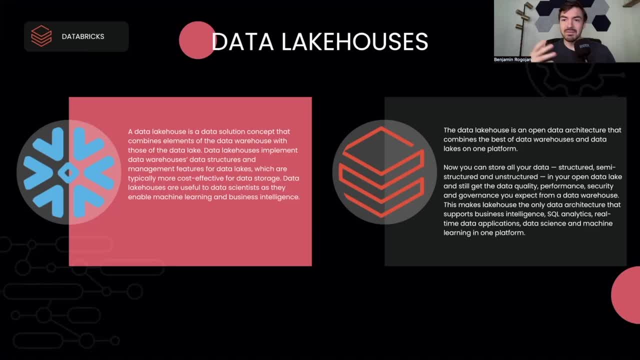 as a combination of data warehouse and a data lake and trying to find the benefits of both: the cost effectiveness of a data lake with the data management kind of benefits that you get in a data warehouse, things like security and just clear table structures that make it easy for analysts and future. 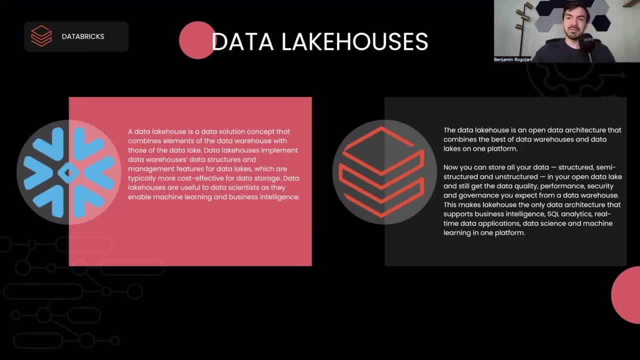 developers to actually approach the data And it's not just a bunch of files that someone's going to have to figure out what exists. where one thing I do think is interesting is Snowflake does seem to try to push more towards the data science use case for data lake houses. 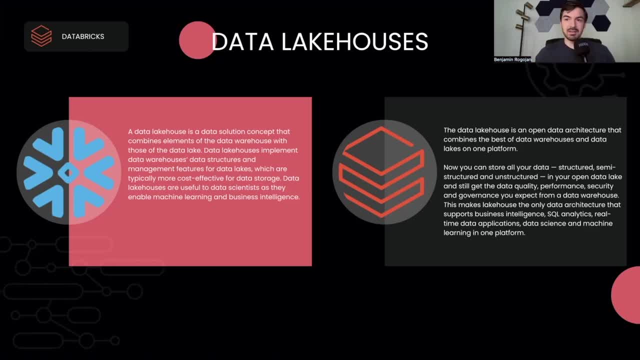 Whereas Databricks is clearly saying: this is everything, This is SQL, This is business intelligence, This is real time analytics. That's kind of the difference that they're trying to sell here. My personal impression of Databricks, which is again: 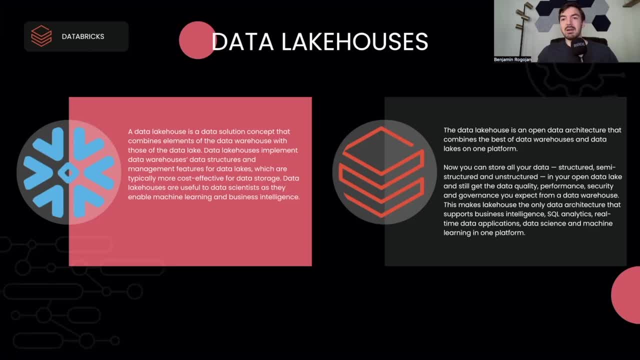 trying to sell more of this data lake house architecture is that it really is geared heavily towards data scientists. It's not to say that it's not built for data engineers, but there's definitely, with everything being focused mostly around notebooks, and we're going to talk about some of the different features that they offer. 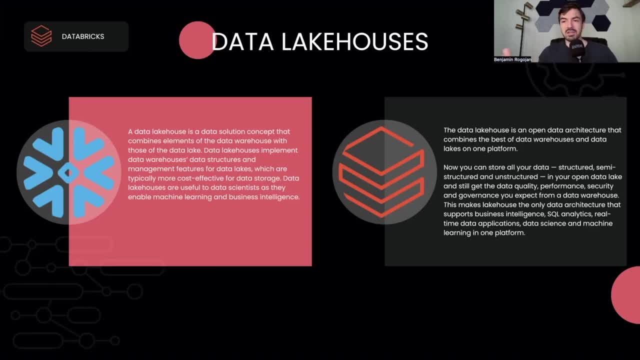 but mostly around notebooks. that's just so quintessential to most data scientists. that that's the feeling I get. There are other things you're going to learn about, such as jobs, such as how you can actually structure tables and stream things, And then there's the idea of data engineering. 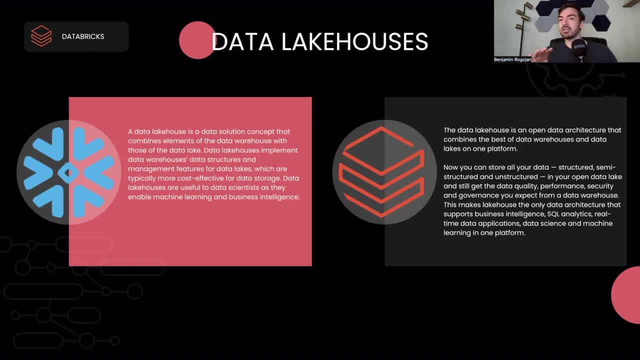 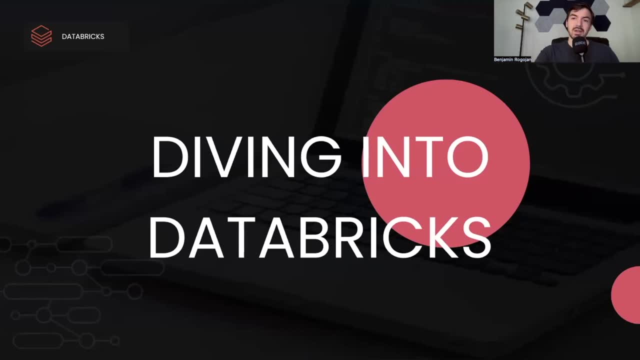 which is a whole bunch of other things that you can do directly from your Kafka instances that do start playing into this whole micro batch, streaming batch, ETL processes that are very familiar to any data engineer. So if we dive into Databricks- and I'm going to just show the kind of key- 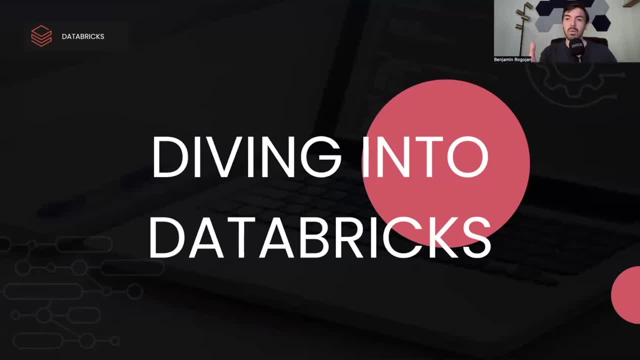 components you're going to work with in Databricks and then we're going to dive right into Databricks, but all of these components are essentially the core tools you're going to use when you go into Databricks. So we're going to have to get used to is the concept of workspaces. notebooks, tables, jobs, clusters and libraries. So we're going to have to get used to is the concept of workspaces, notebooks, tables, jobs, clusters and libraries. So we're going to have to get used to is the concept of workspaces, notebooks. 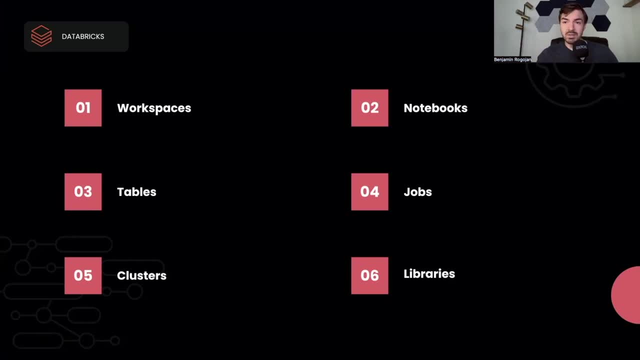 There's a few other kind of components, but I think those are the main ones that if you're a user you have to become familiar with. Tables are interesting because it's kind of this abstraction of often files, But in many ways that's all. tables are in a lot of our modern architecture. 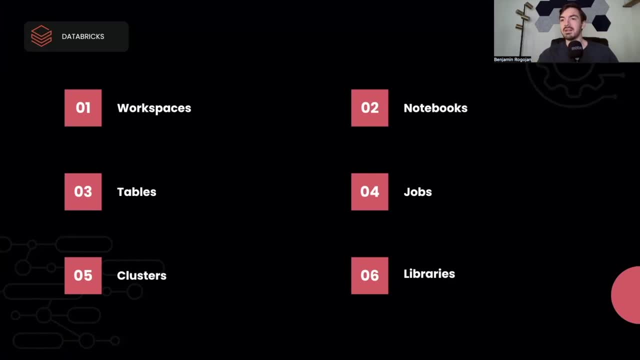 anyways, where there's just kind of the difference between a table and a file is diminishing and schema is really becoming more and more on read, even in the Snowflake world. So let's dive into Databricks itself. So diving into Databricks UI. 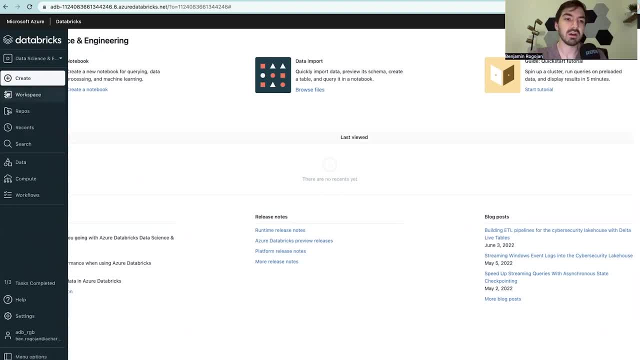 we're going to go into some of the different components that are referenced earlier. Workspaces, I think is decently self explanatory. This is going to be the space that you work. You can either be a specific user or you can create a shared workspace. 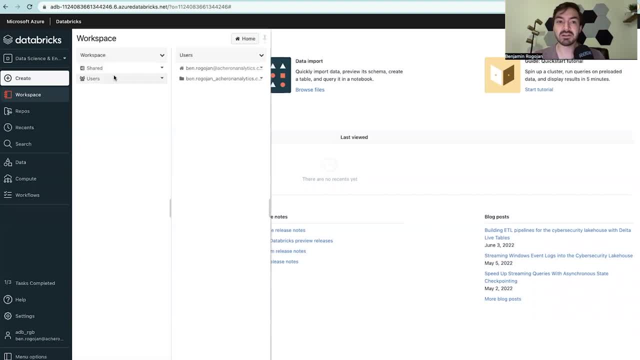 So if you have a team, you can create the shared workspace, Or if you're just by yourself, you can create a user workspace. Next, you can kind of see a lot of what you can do in Databricks using the create button. 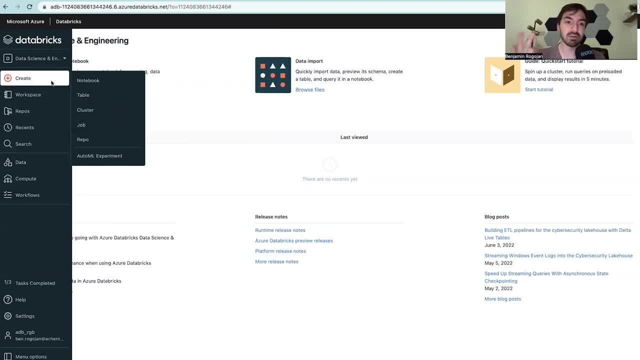 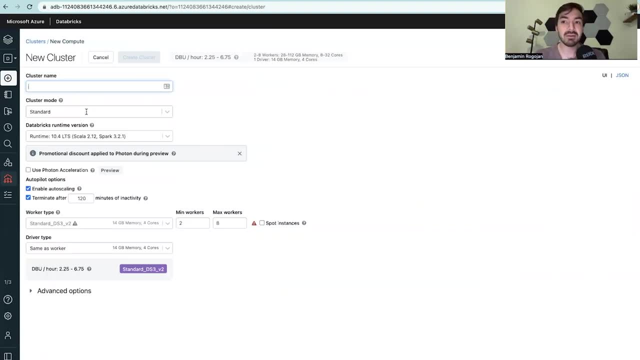 So the create button basically lets you see that you can create notebooks, tables, clusters, jobs and a repo- Clusters- generally pretty self explanatory, If you understand Spark. basically it's the amount of compute. Essentially, you can think about it as that you're going to select in terms. 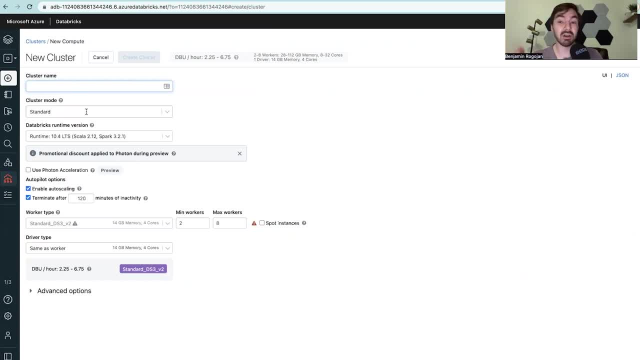 of how many workers you're going to have, in terms of how large the machine is that you're going to use. So, for example, here, if I create a test, you can have a standard machine. You can also work in terms of either having single node or high concurrency. 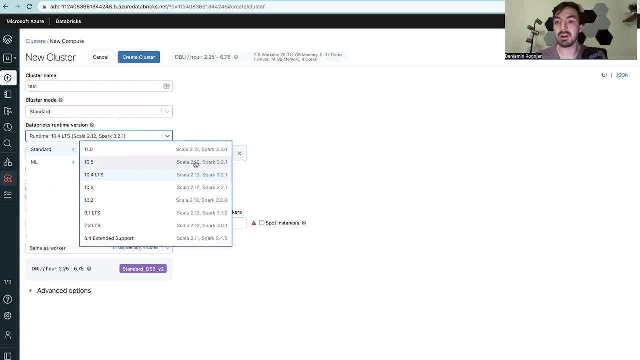 You can then select your Spark version. So more than likely you want to pick whatever Spark at the time is fully supported And from there you can pick how big your machine is going to be. Obviously, the larger your machine, the more data you're processing. 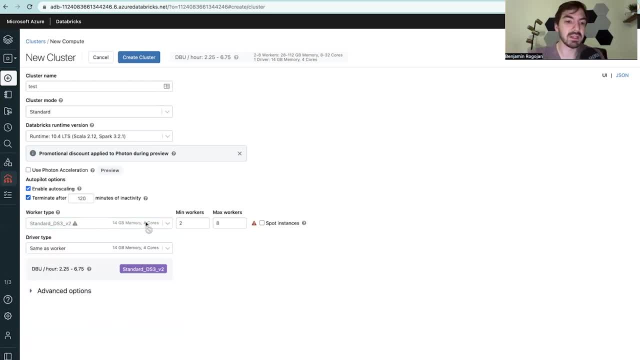 the more expensive it's going to get. So for now, keep it as small as possible. You can also set it to terminate after inactivity, which is great, Again trying to reduce costs if you're not using your machine, And then from there you can just create cluster. 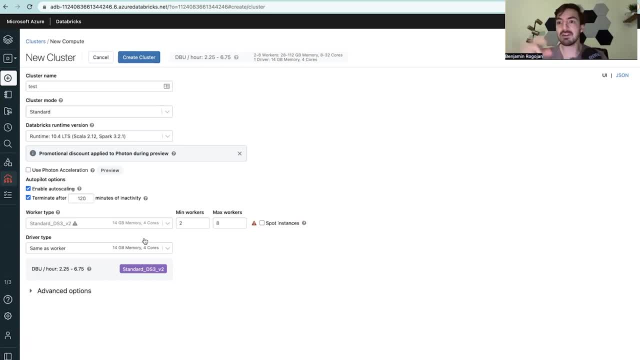 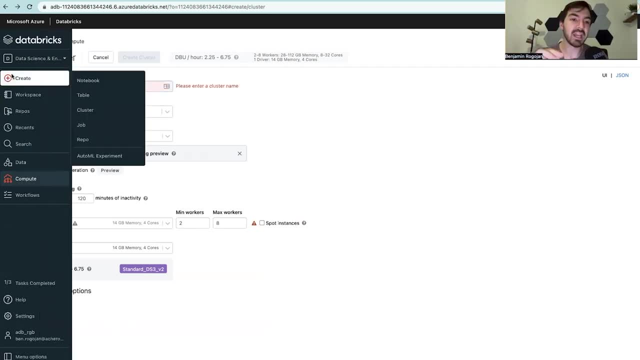 And then in the future, as you're developing different notebooks or jobs, you can tell it to point to different clusters as you go along. Next, let's go over Tables. So this is kind of what it sounds like a little bit. 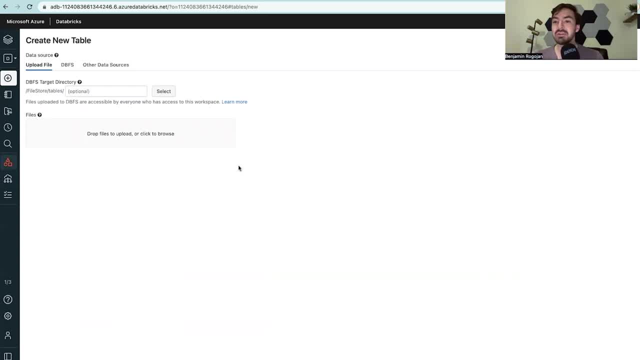 The interesting thing here is that you are going to be dealing with tables at the abstraction of almost pretty much a file which essentially is in a data lake or a data lake house kind of. the context in which you do deal with tables, anyways, but it really kind of, I think, makes it very clear that that's where. 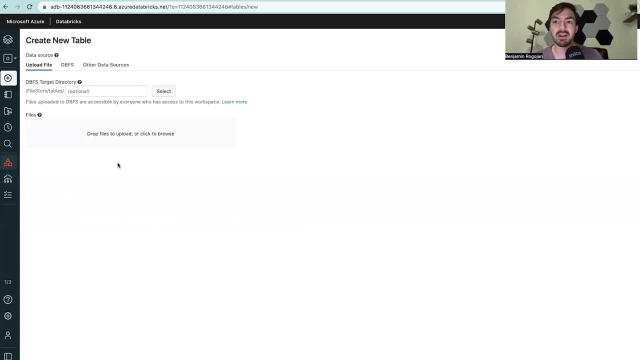 you're dealing with things here, So you can either just upload a raw file like a CSV here, or you can pick a data source So you can pick something like Azure blob storage. You can do S3 if you're using AWS, but I'm using Azure. 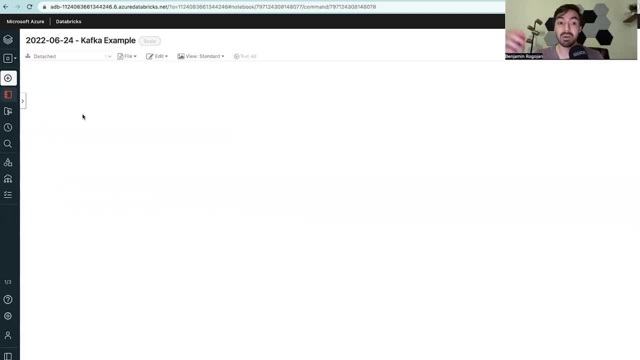 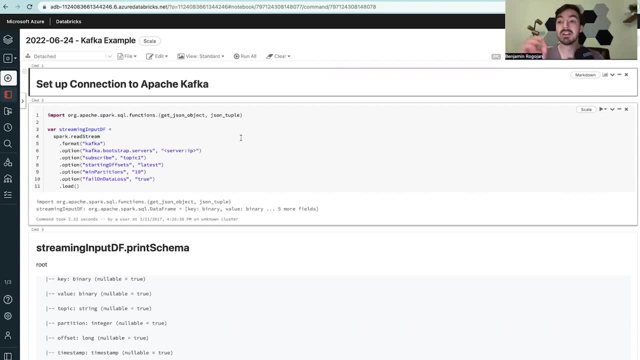 You can pick Kafka And from here you can actually create a notebook to see how it will import said table. Now, with tables, it's important to understand that there's different abstractions of tables. Some can be external, some can be internal, some can be backed by Delta. 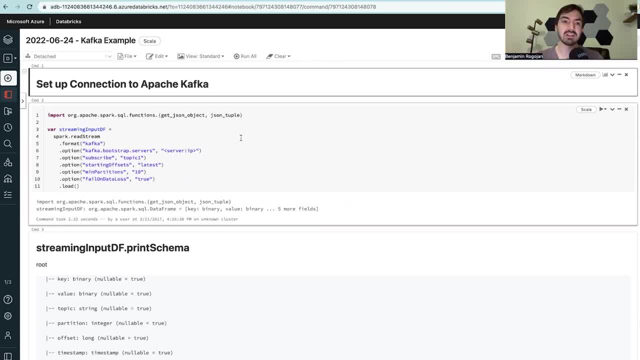 Delta Tables gives you a lot of the benefits of, like asset transactions and things of that nature, whereas normal tables will not, And there's also again more to do in terms of like internally, externally, manually managed, and I'll put up a quick chart here to show all the differences. 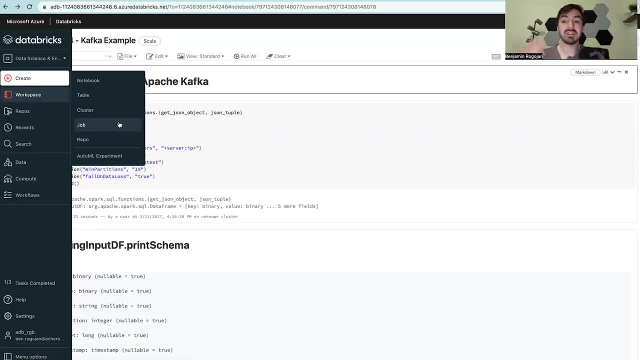 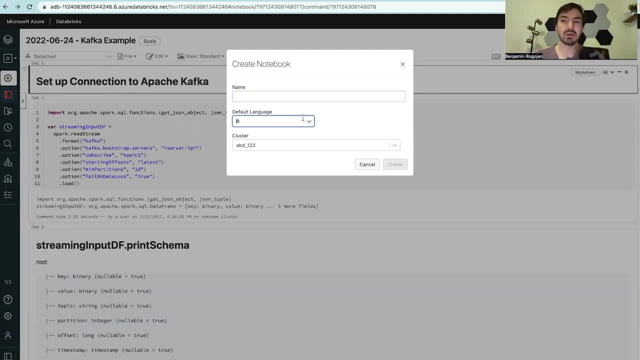 between different types of tables in Databricks. Once you've created a cluster and a table, you can more than likely now go into notebooks and create some sort of notebook, And the great thing about Databricks is it gives you a few options in terms of what. 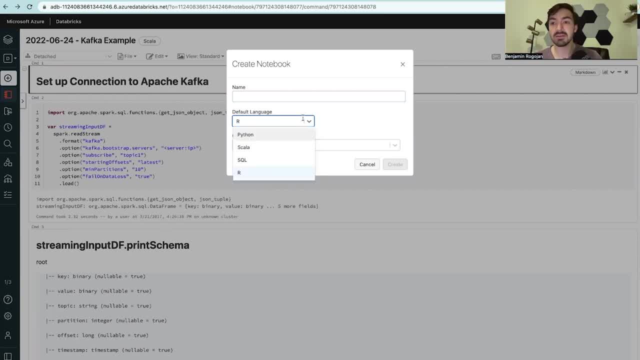 type of coding language you're going to use in your notebook. You can use Python, Scala, SQL or R, So let's just do R test. Yeah, let's just do R test. So we're going to create this on this cluster that I have, and this will. 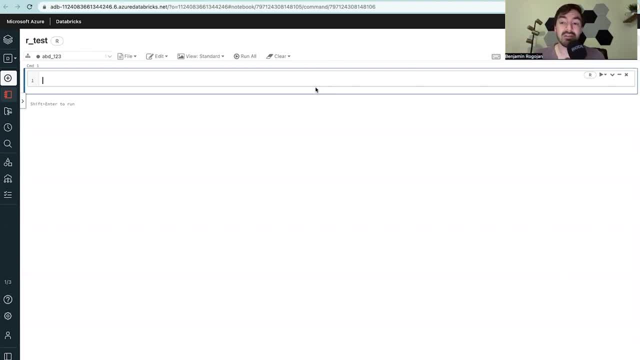 create a notebook that you can work on. And here's where things get even better is a lot of data. scientists often wonder: how do I actually put those notebooks into production? And it's ready for production. You can go to create, you can hit create. 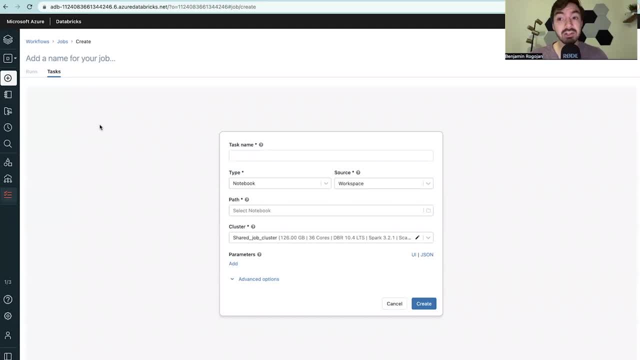 hit job and now you can actually take that notebook and make a job. So if we go here- whatever we can call this R test task- we can select the notebook by going to my users R test confirm. From here we can just hit create. 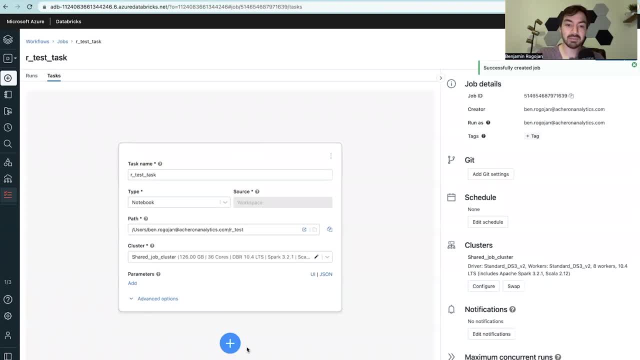 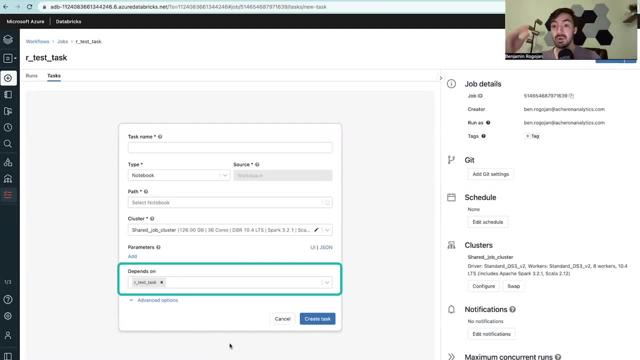 And what you'll see here is that it not only lets you kind of create this task, but you can create more by hitting this plus button, which will then, if you hit plus, create a dependency. So for people who are trying to figure out how to create dependencies, or just 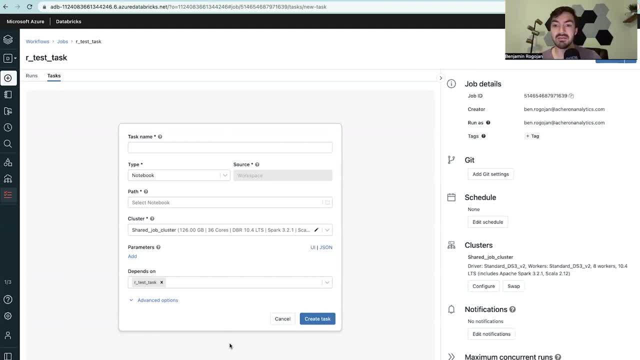 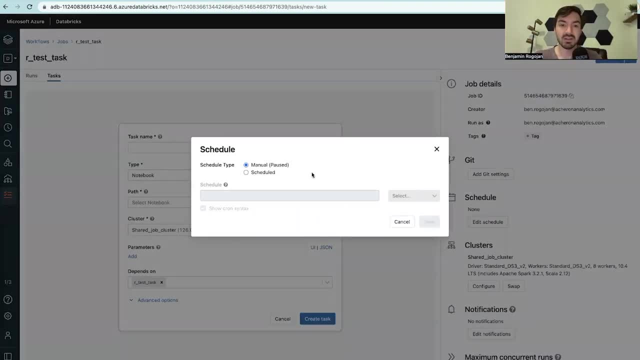 their general jobs anyways. this is one thing that Databricks will take care of. Not only that, it will let you again hit schedule so you can decide when you actually going to schedule that job to continue scheduled. You can set it to some sort of timing, and that can be. 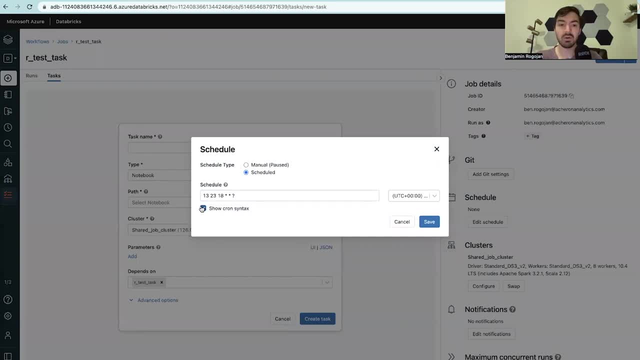 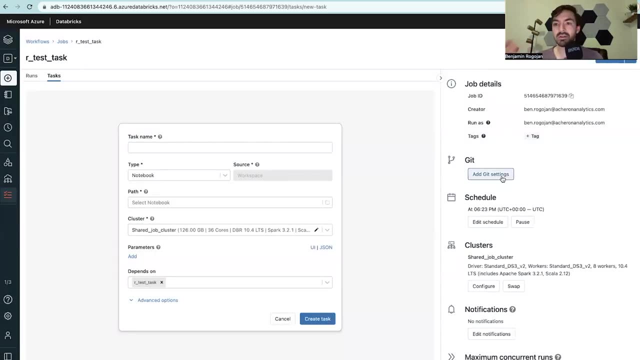 very helpful and for people who want to do a more complex set of timing. you can also use Cron. you can hit save to schedule that job. You can also then connect with Git. So if you want to have some form of version control, 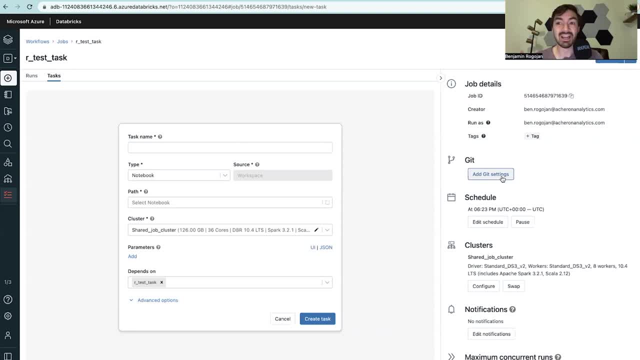 that is also automatically integrated to all of Databricks. Again, this is something that I really do enjoy about the Databricks kind of developer experience is that so much of it is integrated, and I do kind of wish Snowflake was a little more like that. 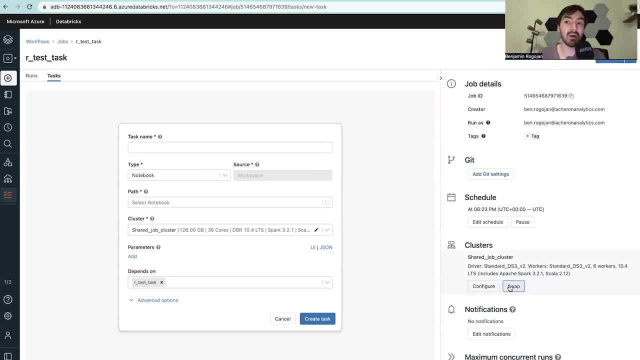 where a lot more of your workflow was integrated into one, And you can also swap out whatever configuration of Spark cluster you're using. So if you're deciding that this is no longer sufficient, or maybe it's too much in terms of cluster size, you can resize that and fix that. 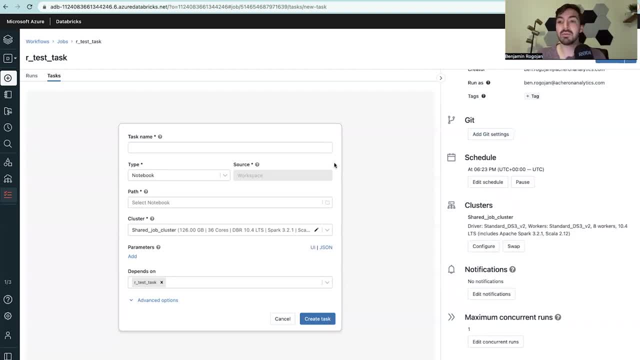 So that's really what's great about jobs: It allows you to basically take a notebook and essentially truly productionize it. All these components are really great because they make data science workflows, I think, much easier to productionize. If you are really comparing Databricks to Snowflake. 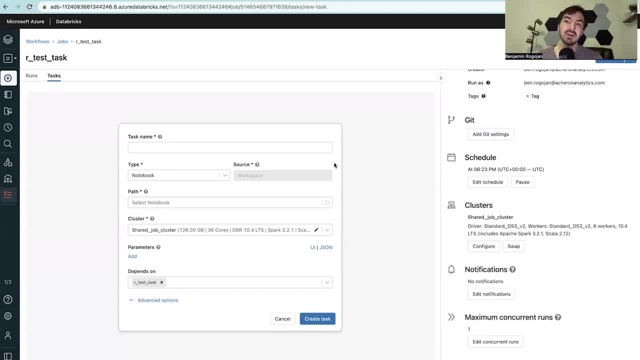 you're not going to get that in the current setup of Snowflake- And I do think Snowflake is trying to add more with a lot of their ability to start running Python on your data. But in terms of native functionality, the fact that Databricks use Spark as their underlying processing engine is what 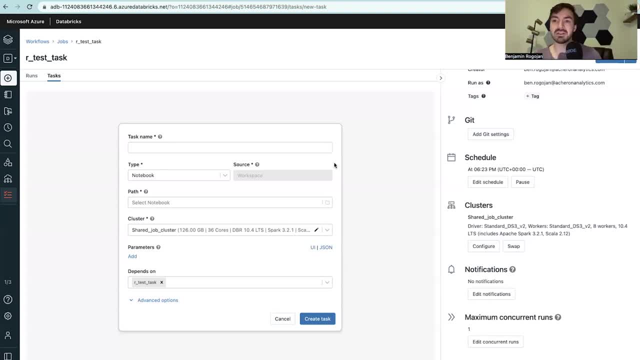 gives them this ability to run multiple different languages in terms of jobs and notebooks, as well as gives them this ability to kind of create jobs in this way. You do have tasks in Snowflake, but I really always kind of wish that those tasks were somehow more like this. somehow I could actually see them in a UI. 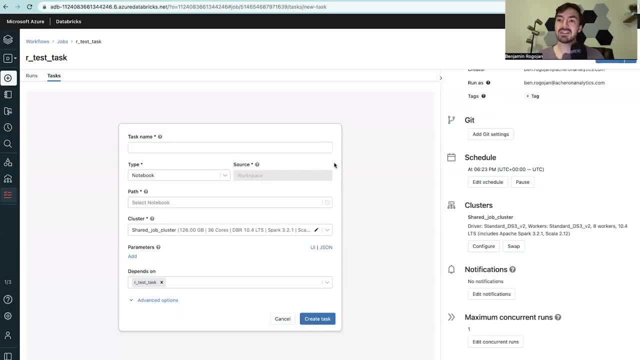 create them rather than having a purely SQL based approach. Anyways, guys, this is your intro to Databricks. If you enjoyed it, let me know in the comments below. Maybe I can start creating a few jobs here if you guys are really liking it.